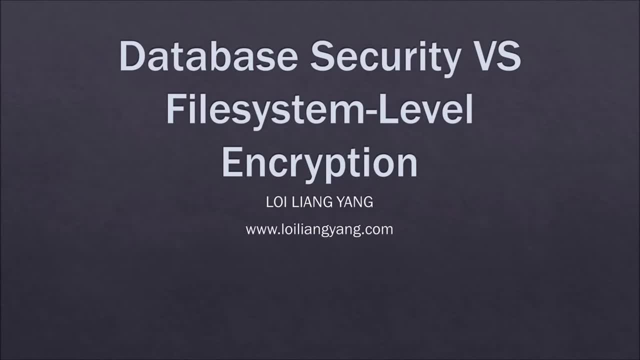 Today we will be discussing on the different types of security mechanisms to help protect databases. There are two primary ways to encrypt database content: either through the database encryption itself or through the file lever encryption. Databases have encryption capability by default using a well-known encryption method called. 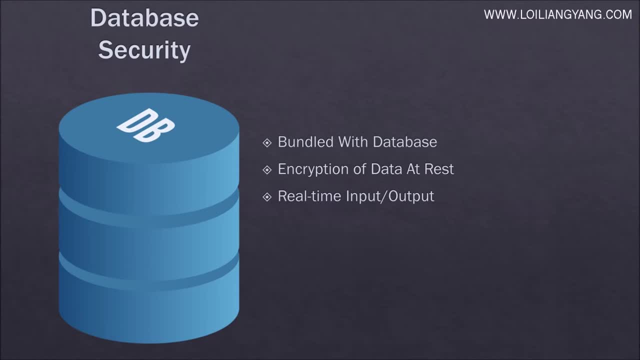 Transparent Data Encryption. It is usually bonded with the database and allows encryption of data at rest. Furthermore, the encryption occurs immediately during input and decryption on output, therefore providing greater security defense against unauthorized access. For example, a hacker gained access into the database system and he is going to query the 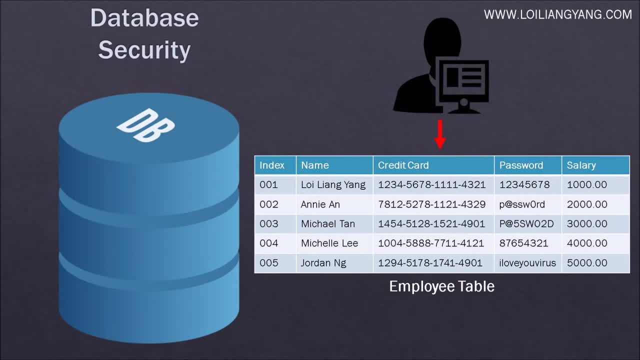 employee table. If there are no security mechanisms in place, he would be able to see all the information in the employee table, including credit card number, salary, password and the likes. Databases are the best place for hackers to access into because the data are highly structured. 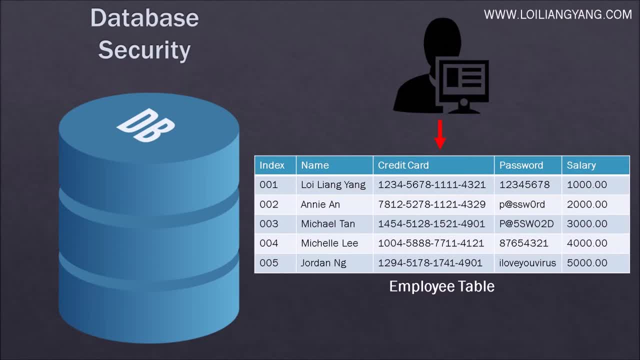 and organized. Furthermore, sending a SQL query is extremely simple and straightforward, making the attack much quicker. One technique is to mask the information. For example, the hacker accessing the information of the credit card will see the credit card section is populated properly, But the reality. 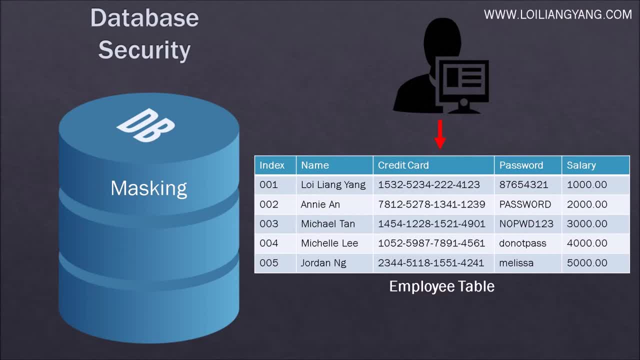 is that the information has been substituted by the system. At the same time, the same masking is performed on the password column of the table. This allows the information to appear as normal, but in reality it is worthless data that looks valuable. Another form of database security is redaction. Redaction hides certain areas of the table. 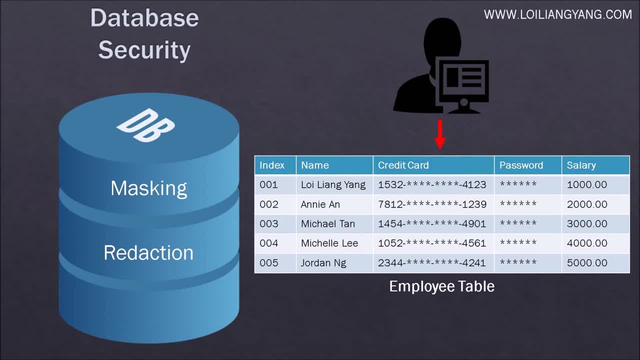 column. In this example, the hacker can see only the first four digits and the last four digits of the credit card number, Also making the column practically worthless. At the same time, the password is also being redacted to show only asterisk, Again removing the ability for the hacker to see any valuable 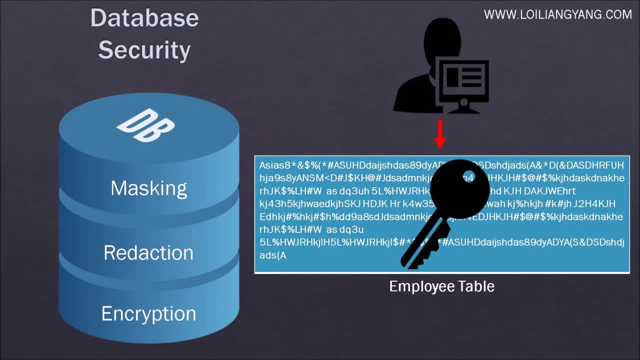 information. Another very important technique in database security is encryption. If a hacker enters into the database, he will not be able to see any form of information at all, because it requires a key to decrypt the information into human readable content. An encryption by itself is a huge security domain in the field of cybersecurity. 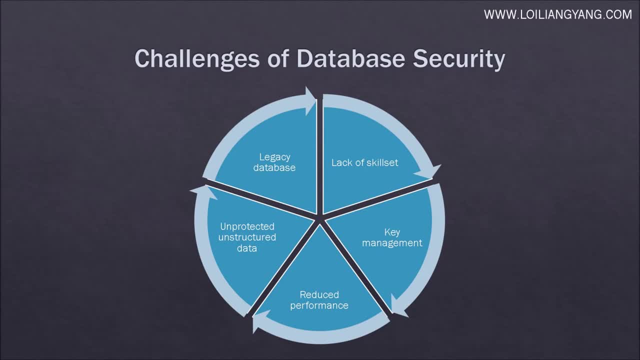 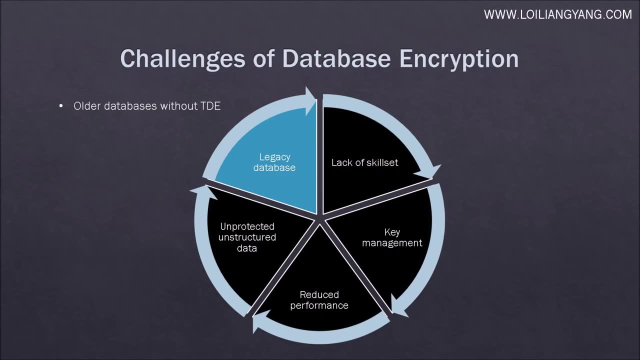 And there are many challenges with securing databases using database security mechanisms. Many enterprises support older database versions that do not include TDE functionality for database protection. It can be difficult or impossible to migrate these older database versions to more recent versions offering TDE database encryption. given the constraints of the package, 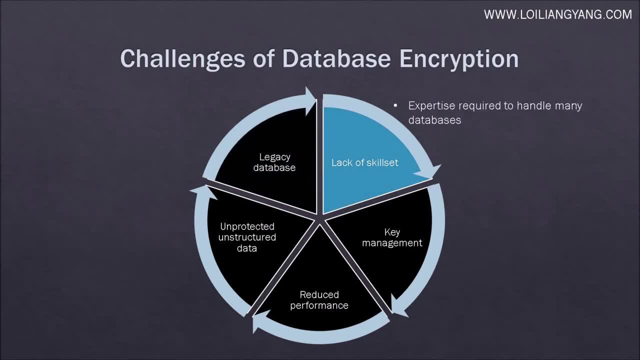 application. There is also a huge lack of database experts in the market who not only have depth in a single database type. they need to have breadth with all flavors of databases. There is SQL Server, NoSQL, MariaDB, MongoDB, DB2 and so many other types of databases that needs. 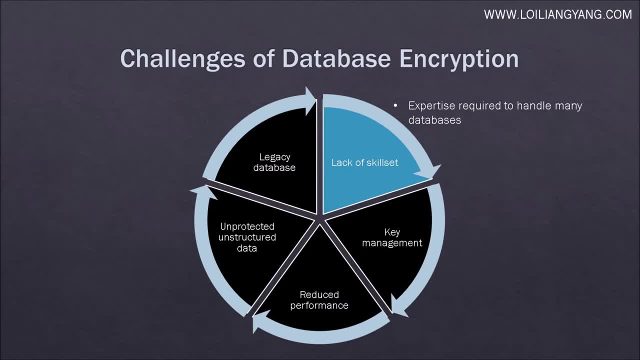 to be supported in order to ensure consistent security settings. With database encryption, there is a need to manage the encryption keys. This introduces another huge headache because there can be multiple types of databases with many different instances in which each have a key or multiple keys involved in order to secure those databases If the key falls. 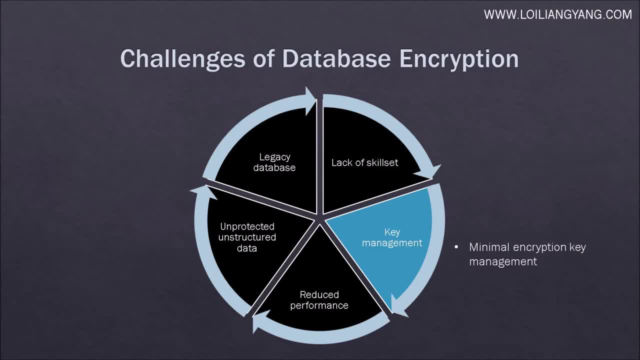 into the wrong hands or is mismanaged, a lot of very sensitive information can be gone forever. Database encryption also introduces performance issues. The first issue for database encryption is performance. The problem is that the data is not well managed. The data is not well owned. The data is not well managed. the data is not 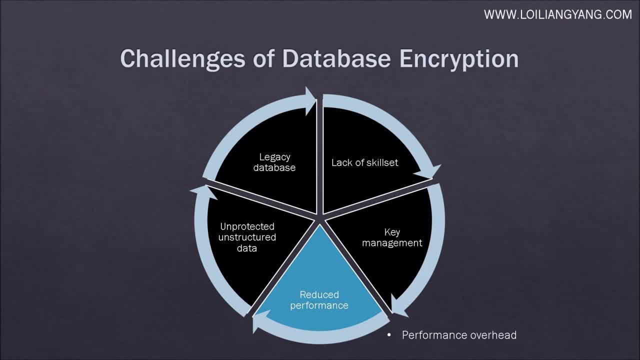 because encrypting and decrypting data can cause high CPU usage. This is crucial to database performances for transactional systems. There are many other types of data surrounding structured database data. There are backups and archive files residing in the database server and there are very 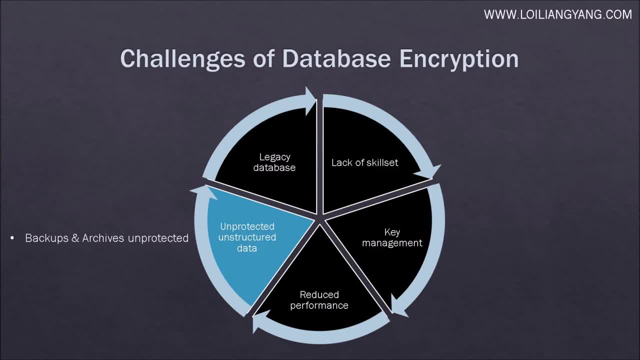 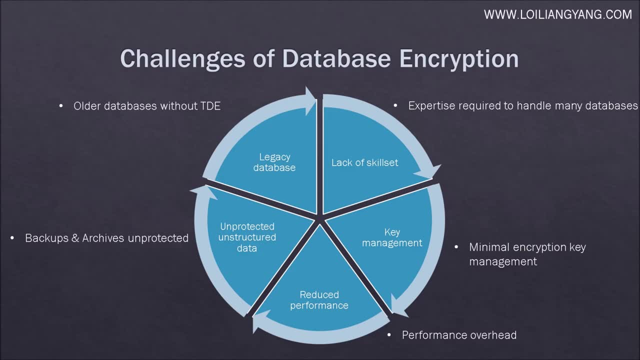 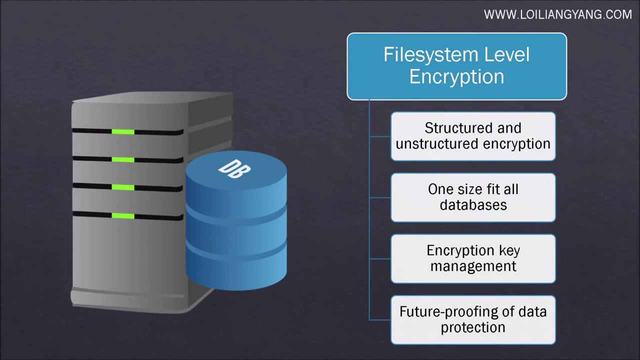 little protection mechanisms available to secure these important files. Looking at so many challenges faced by the security systems in the database servers, we need to look elsewhere. File system level encryption, often called file or folder encryption, is a form of disk encryption where individual files or directories are encrypted by the file system itself.